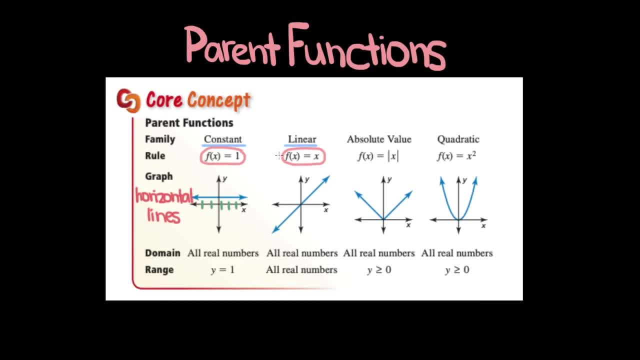 then the output will be that same value. So, for example, let's say we set our input x to be equal to 1, then our output will be 1 as well. The most important characteristic of linear functions to know is that every unit increment in x will result in the same change in y. And to put this: 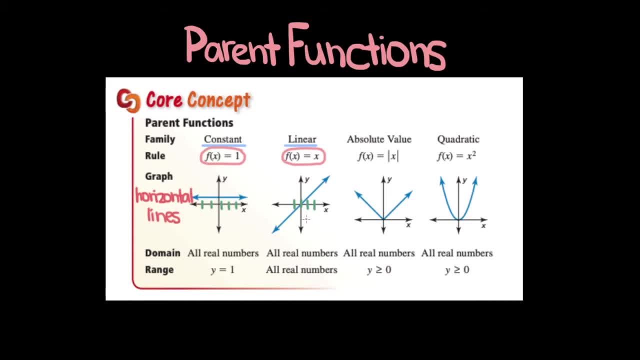 characteristic into more mathematical terms. we're going to need to calculate the value of x, So let's start with the first family of functions, which is f of x, which is the absolute value of x. We refer to this as having a constant slope. 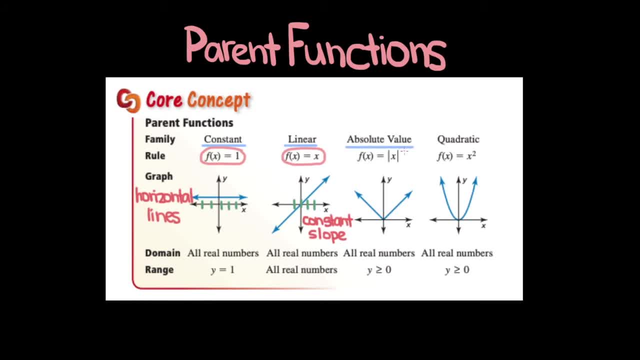 Now let's move on to the absolute value functions. In this case, the parent function is f of x is equal to the absolute value of x, And from the graph we can see that the range of this function, that is, the output, is always positive, because absolute value, by definition, is just the magnitude. 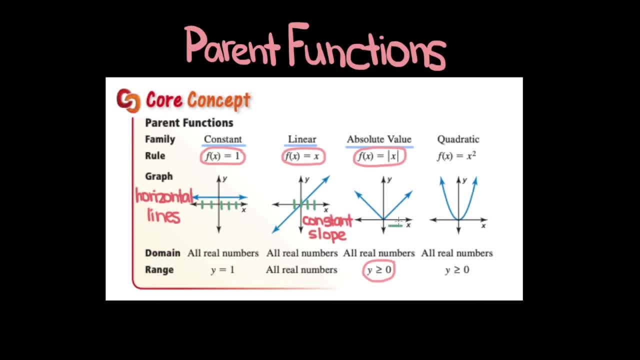 of a number, You discard its sign And so, as you can see on this graph, positive x values correspond to positive y values, but then negative x values correspond to positive y values as well, because we're discarding the sign And because of this, all absolute value functions will be v-shaped. 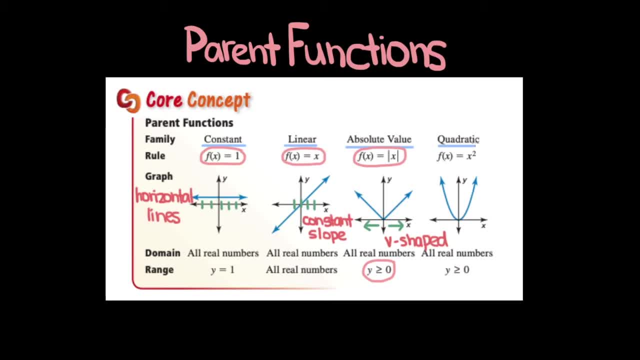 The fourth and final family functions we're going to be talking about are quadratic functions. In this case, our parent function is f of x is equal to x squared. So you input a value of x and the output will be that value squared. 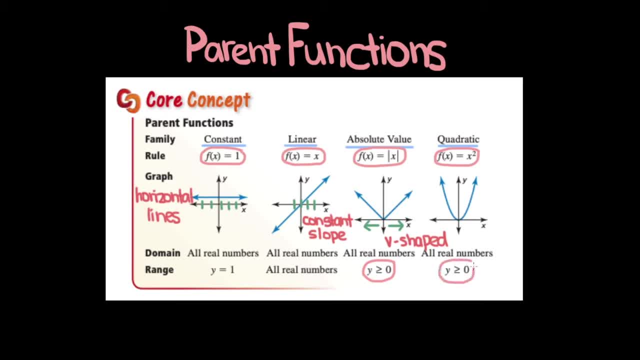 For this particular function, y is always positive because the square of a number, whether it's positive or negative, will always be positive For quadratic functions. every unit increment in the positive x direction will result in an increasing change in y And, as a result, all quadratic functions will be. 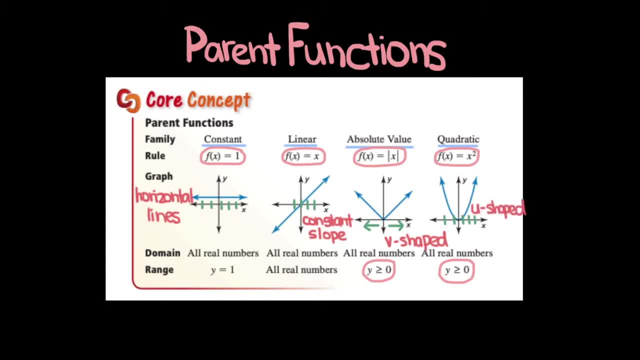 u-shaped. Now, these are four relatively simple types of functions, and we'll be getting into more of them later on in this course. Now let's move on to transformations, which will be the focus of the rest of this video. Essentially, transformations are ways we can alter or manipulate these basic 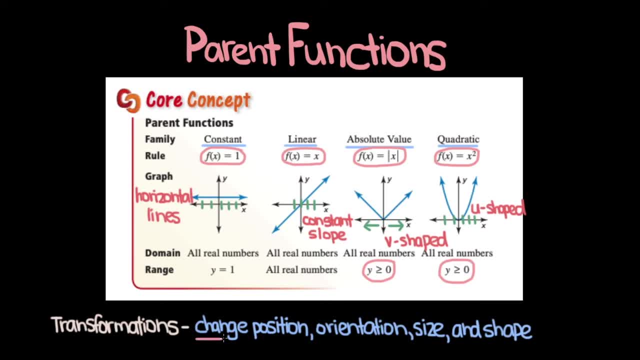 parent functions. In transformations, we can change the position of our function on the xy plane. We can shift it in the horizontal direction or the vertical direction, and these types of shifts are known as translations. Now we could also change the orientation of these functions In the case of the absolute value or 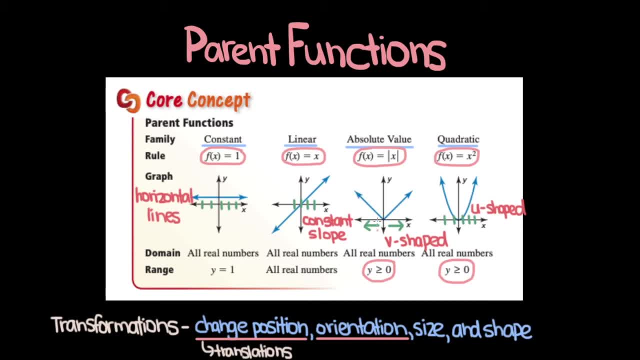 quadratic functions. we can alter whether they open up or down and things like that, And changes in orientation are known as reflections, And we can also alter the size and shape of a function by structuring it. For now we'll focus on translations and reflections. 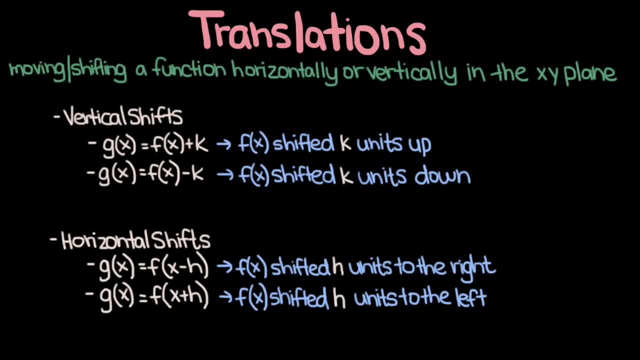 and I'll cover stretching and shrinking in a future video. Let's start off by going over translations. Like we mentioned in the previous slide, translations are a type of transformation that involve moving or shifting a function horizontally or vertically in the xy plane. So we can break down translations into vertical shifts or vertical translations. 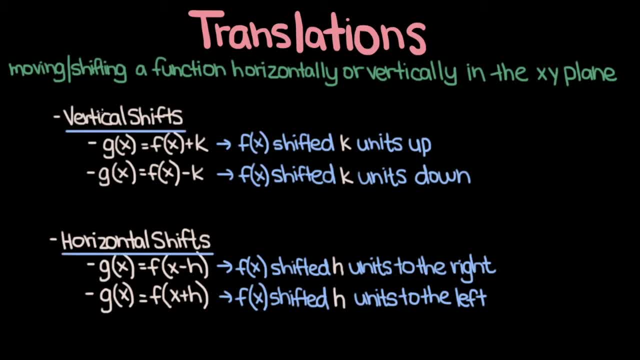 and horizontal shifts or horizontal translations. Vertical shifts are a little bit easier, so let's start there. Essentially, if you have some function f of x and you define g of x to be f of x plus k, then what g of x is is f of x shifted k units up. And similarly, if you define g of x to be f of x, 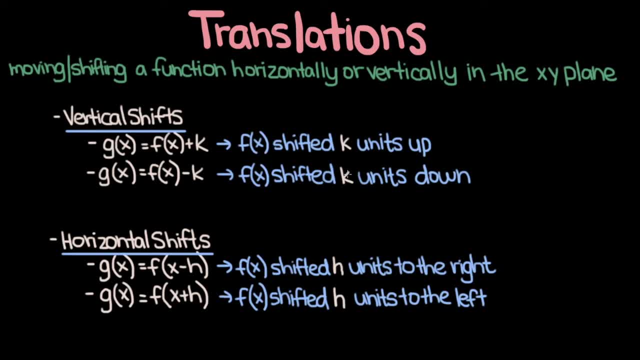 minus k, then g of x is f of x, shifted k units down. So when we're adding the constant we're shifting up, and when we're subtracting a constant we're shifting down. So let's do an example of this. Let's say f of x is equal to x squared, So we're dealing with the. 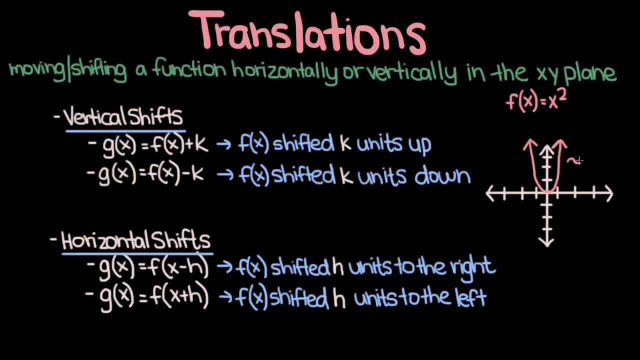 parent function for a family of quadratic functions. Okay, so here's f of x graphed, and now let's consider what g of x, which we can define as f of x plus 2, so x squared plus 2, let's consider what g of x would look like in relation to f of x. Remember, since we're 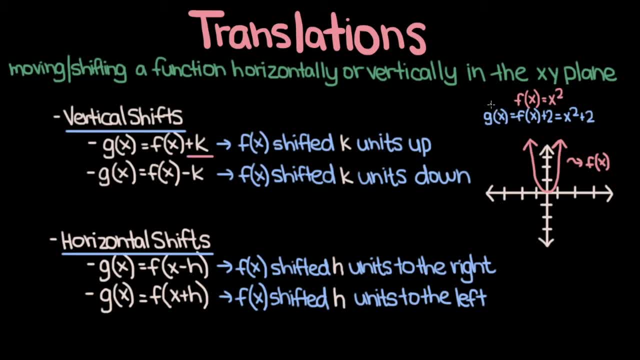 translating, the shape of the function is not going to change, but the position is: We're clearly dealing with some sort of vertical shift here. clearly we're dealing with some sort of vertical shift here. g of x is in the form f of x plus k, and k is 2, and so g of x is going to be f of x. 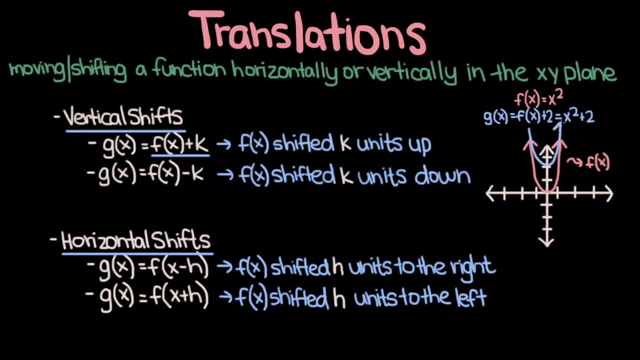 shifted two units up is going to look something like this: And if you want to think of it this way, for every point x comma y on our curve f of x, there is a corresponding point on the curve g of x where the x value is the same but the y value is the y value for f of x, so y. 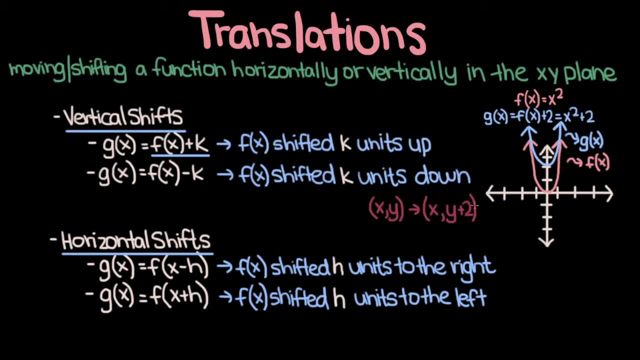 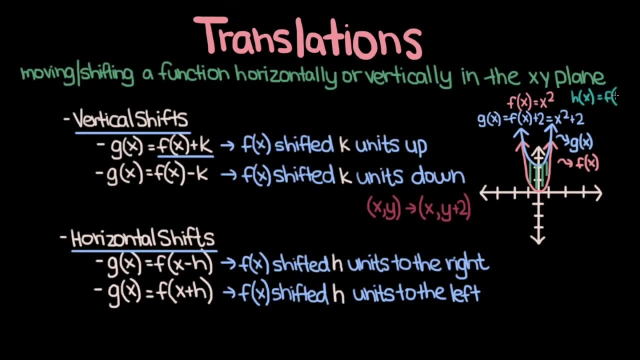 plus 2.. And so this corresponds to the shifting of the graph two units upward. Now, visually, the 2 in this sort of diagram is the vertical distance between the two curves at any x value. Now let's say we have a third function, h of x, which is defined as f of x minus 3, so x squared minus 3.. 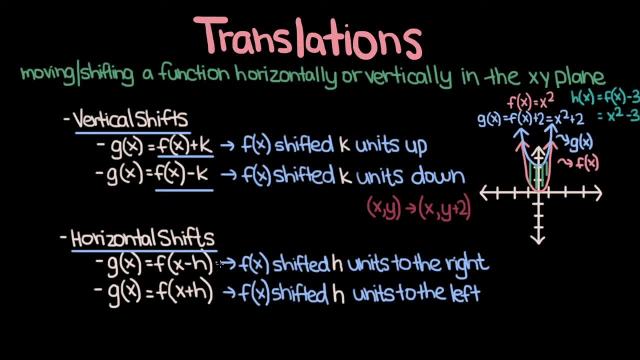 This is still a vertical shift, but now we're shifting in the negative y direction, since k is negative. Specifically, we're shifting f of x three units down, and so h of x would look just like f of x, except now all its points would be shifted three units down. So if we think about starting at the vertex, the vertex is at zero, zero. 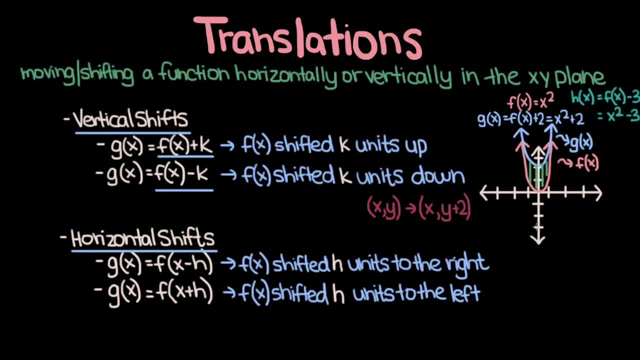 and f of x, and so h of x would have a vertex at zero negative three. so it would look something like this. And that's really all there is to know about vertical shifts. Now let's get into horizontal shifts. So once again, if we have a function f of x and we define g of x to be f of, 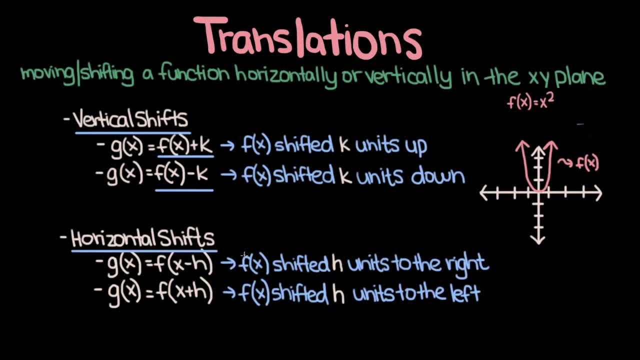 x minus h, then all g of x is is f of x shifted h units to the right. and if we have g of x defined as f of x plus h, then g of x is just f of x shifted h units to the left. Now the one thing. 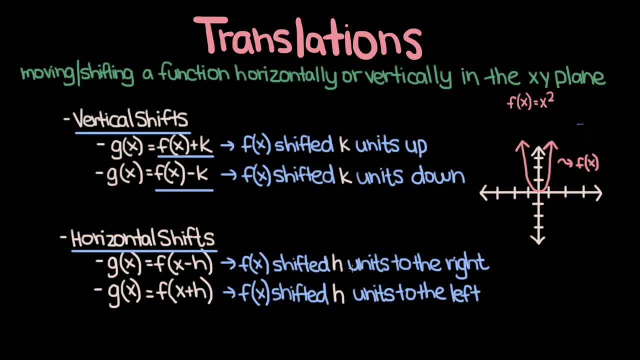 that's a little bit not intuitive about horizontal shifts is that the direction of the shift is opposite to the sign. So, for example, if we consider this second case, where we have f of x plus h, we typically associate the plus sign with moving to the right. 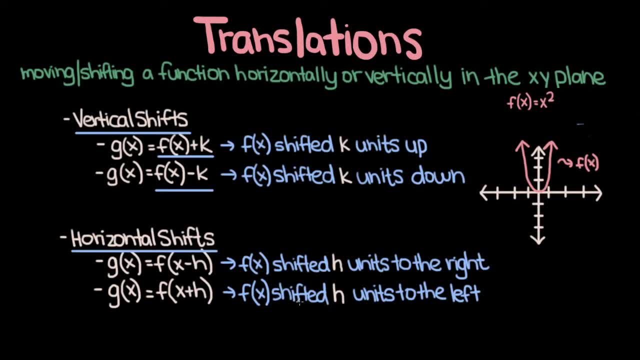 turns out that this actually means f of x is shifted h units to the left. So that's just something to keep in mind. Let's start off by considering the case where we have the function g of x and we define it as being f of x minus 2.. So in other words, if we plug in x minus 2, 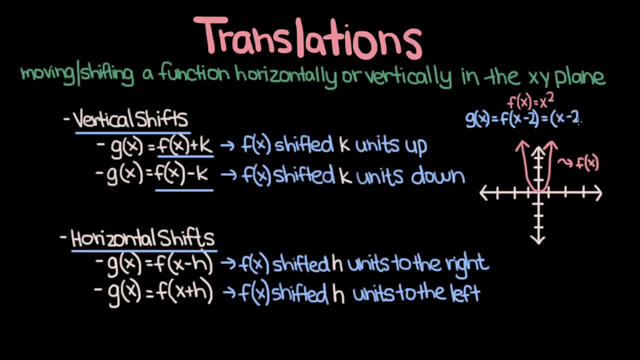 into our function f, we get x minus 2 whole squared Now, just based on our definition, because we can see g is in the form f of x minus h. where h is 2, we know that the function is going to shift 2 units to the right. but let's just think a little bit about the intuition behind that. 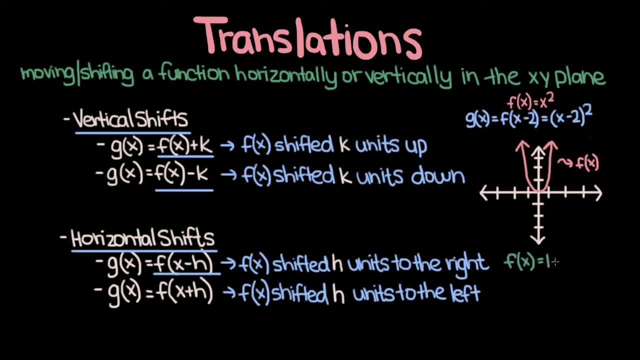 Let's consider when f of x is equal to 1.. Now f of x is equal to x squared, and so f of x is going to be equal to 1 when x is plus or minus 1, and so the two points we're looking at are negative. 1 comma. 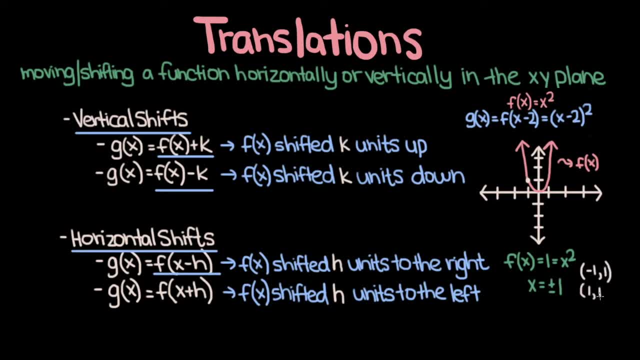 1, which is here, and 1 comma 1, which is here. Now let's consider the points where g of x is equal to 1.. So f of x is x minus 2 squared, and we can see that x minus 2 whole squared is equal to 1. 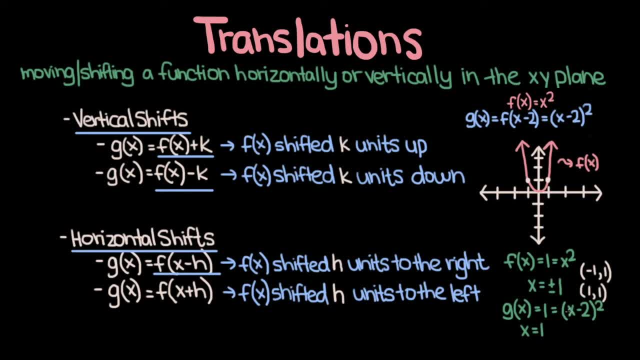 when x is equal to 1. in the case you get 1 minus 2, which is negative, 1 squared equals 1. or when x is equal to 3.. 3 minus 2 is 1 and 1 squared is 1.. And so the points on the curve g. 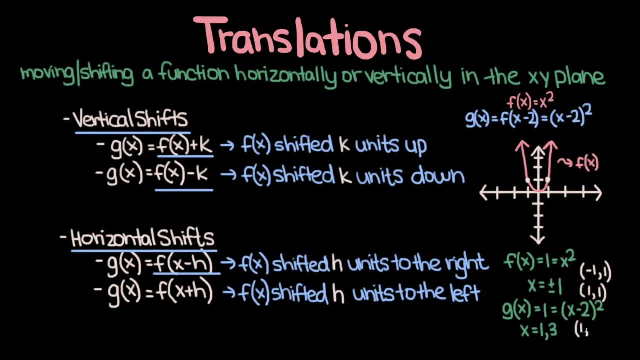 of x, where g of x is equal to 1, are 1, 1, and 3, 1.. And so if I plot those two points, the point 1, 1 was the point we plotted before, so I'll just indicate it with a smaller. 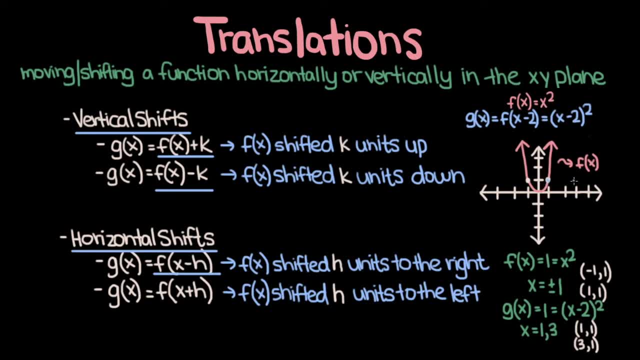 blue circle inside that white circle and the point 3, 1. is this point right here? And notice something special about these two points? let's first consider these two. 1 comma 1 is just the point negative. 1, 1 shifted to the right two units and similarly 3 comma 1. 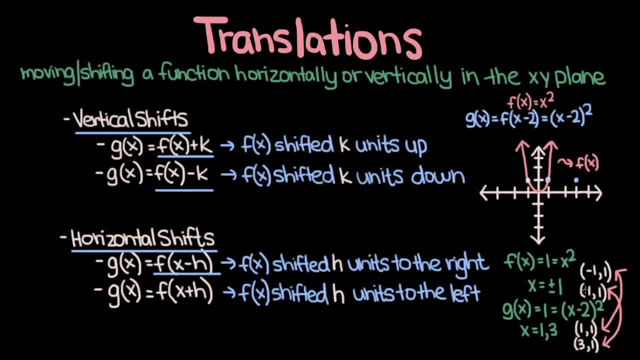 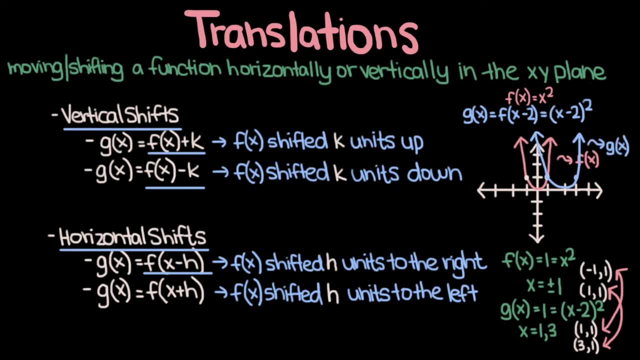 is the point 1, comma 1, shifted to the right two units And if you were to plug in some more points, you would see that g of x looks roughly like this and my x- y isn't perfectly to scale and that's why the shapes of f and g look slightly different. 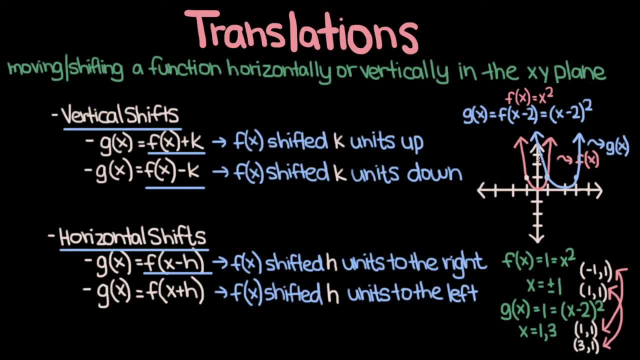 but in reality, the shapes of these two functions are exactly the same, since all we're doing is changing the position, Specifically shifting f. two units to the right will give us g, And so in this case, if we're looking visually, all the two represents is the horizontal distance. 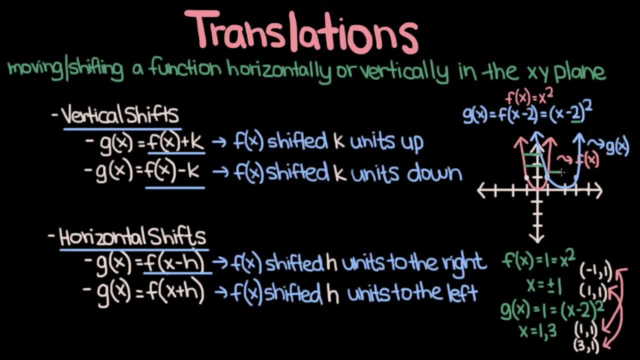 from the pink curve to the corresponding points on the blue curve at any given y value. And of course we can do a shift in the opposite direction as well. Let's say we have a function, h, which we define to be f, so h is x plus three whole squared. and since in this case, 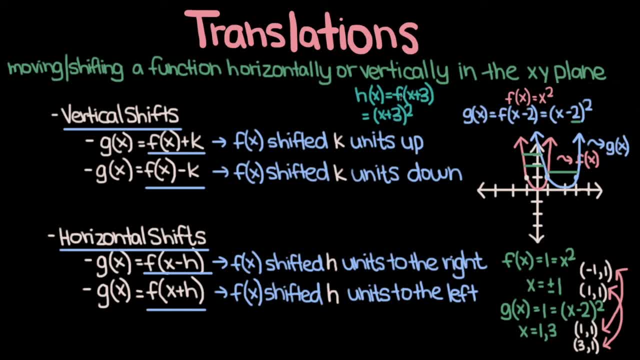 h is positive, we're going to be shifting to the left and, specifically, since h is three, we're going to be shifting f three units to the left to get h, And so h is going to look roughly like this Once again. if you just want to. 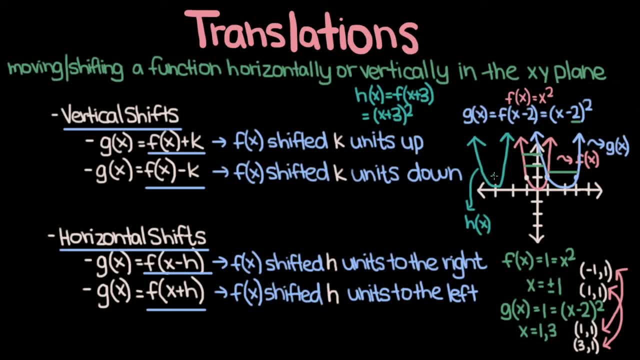 think about this and see what you can do. you can go to our other videos and find out more about the, about the vertex. For f, the vertex is at, and for h, it's been shifted three units to the left, so it's now at. And that's really all there is to horizontal shifts. Now let's move. 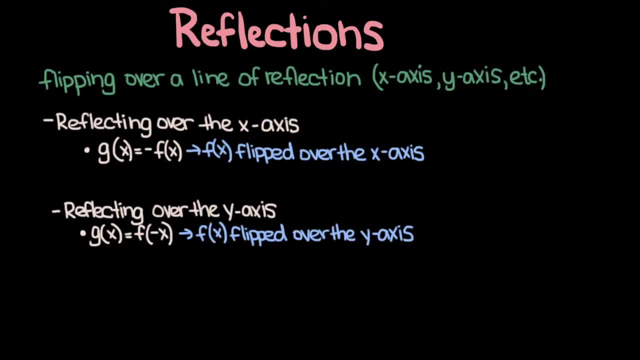 on to reflections. So while translations involved changing the position of a graph of a function, reflections involve changing that graph's orientation. So this could involve flipping the graph of that function over a line of reflection So that line could be the x-axis or the y-axis, or maybe the line y equals x and things like that. but for now we're just 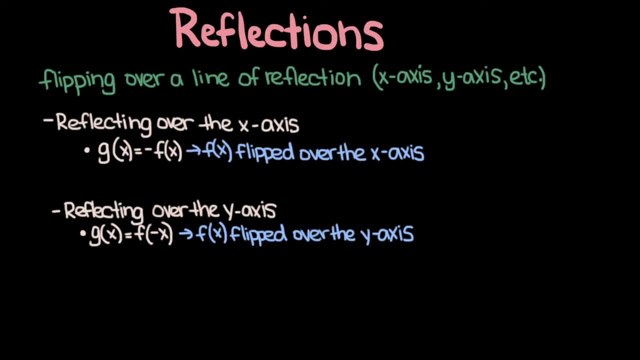 going to focus on reflecting over the x-axis and reflecting over the y-axis. Let's start off with reflecting over the x-axis. If you have some function f and you define g to be negative f, all g is f flipped over the x-axis. So let's stick with f from last time. 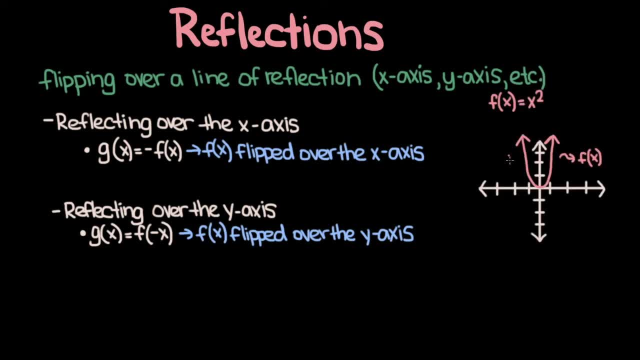 we have, f is equal to x squared. So here we have f graph. as you can see, it's a parabola that's opening upward. and now let's say we create a function, g, which is defined as negative f, so negative x squared. Now, since g is in this form, 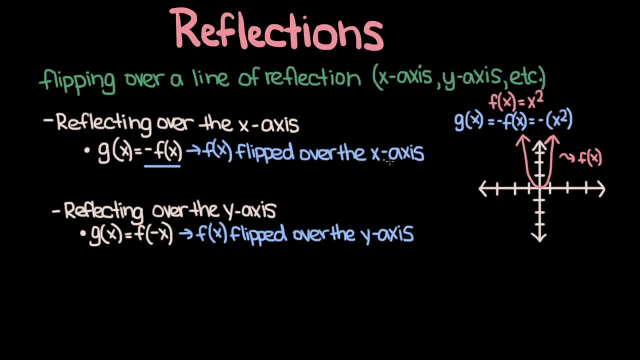 negative f. we know it's just going to be f flipped over the x-axis, which is this line right here. So just imagine you take f and you flip it over that line, and so g is going to look something like this: Once again we're preserving the shape, but we're changing the orientation. The parabola g opens. 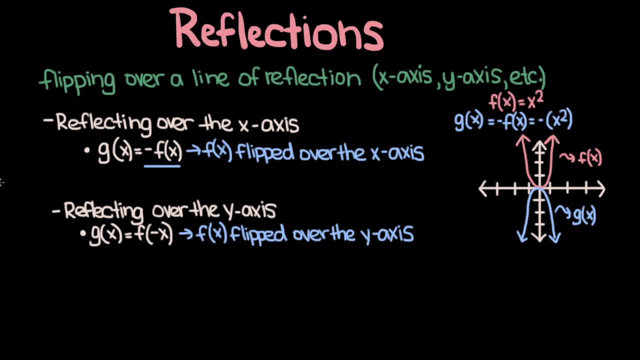 downward, while the parabola f opens upward. In terms of the intuition behind this, consider any point on the curve f. right, Let's say we look at this point again, which is the point Now. let's consider the corresponding point on the curve g. so we're going to plug in. 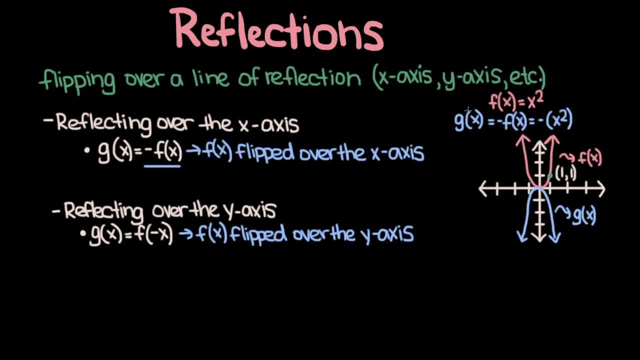 the same input. so we're looking for g, and g is just negative of f, f is 1, and since we have that negative sign, g will be negative 1.. So it's this point right here, and so ultimately, what we see is that all the points on the pink curve get flipped over the 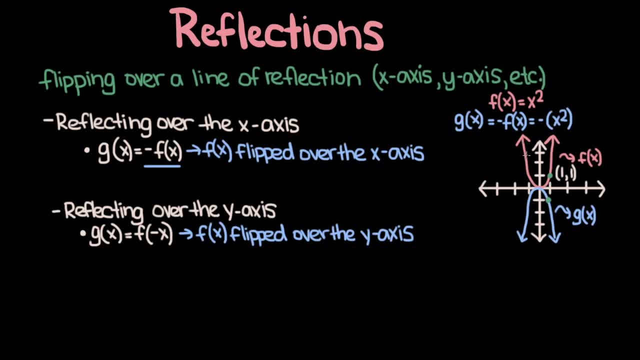 x-axis to form the blue curve and that's really all there is to reflecting functions over the x-axis. Now let's talk about reflecting over the y-axis. So if you have some function f and you define g to be f, then all g really is is f flipped over the y-axis. 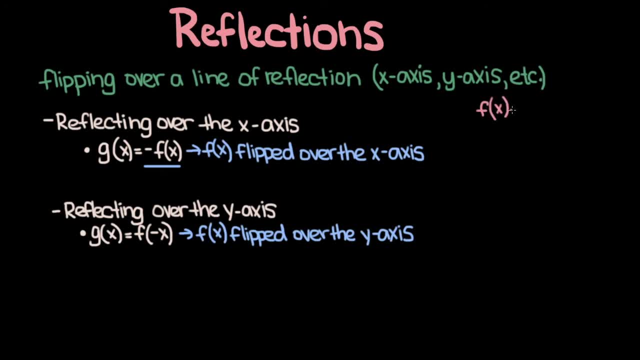 All right. this time, let's say f is equal to x cubed. All right, so this is what f looks like: it's a cubic function. Now imagine that we have a function g which is defined as f. so whenever we see x, 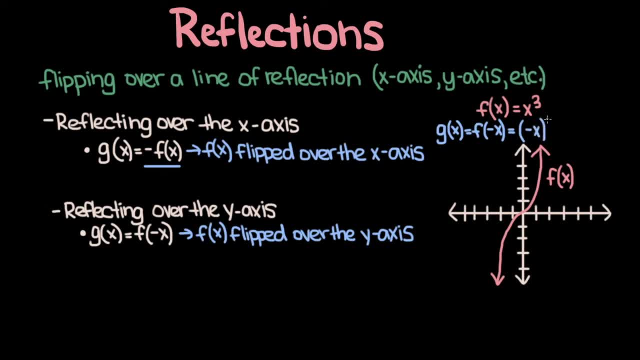 we're going to replace it with negative x, so in this case we would get negative x cubed. So this function is in the form of g is equal to f, and whenever a function is in this form, we know it's f flipped over the y-axis. So it's going to look. 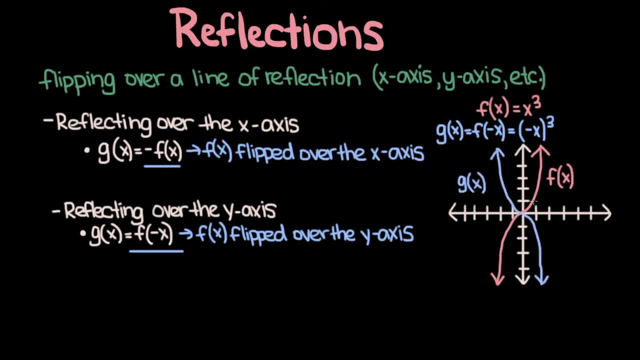 something like this. So, in order to understand the intuition behind this, let's consider the point which is on the curve f, and now let's think about the corresponding point on the curve g. The corresponding point on g is going to be negative: 1 comma 1,. 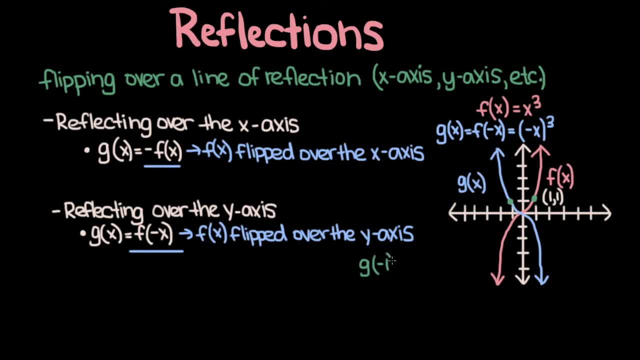 because when we pass in negative 1 to g, we get g which is equal to f, of negative, of negative 1, which is equal to f. So we see that f is equal to g. but also in general we can see that. 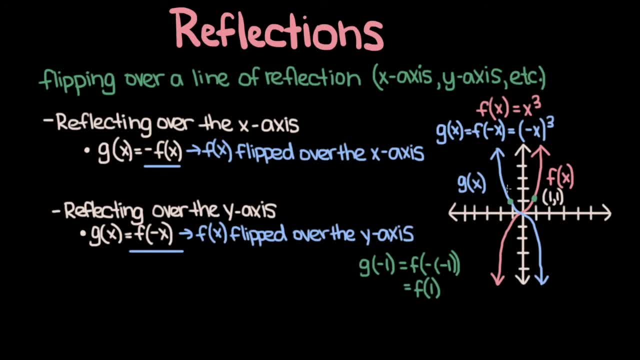 f and g have the same y values when their x values are of opposite signs, and this explains why g is f-reflected over the y-axis, and so hopefully this intuition made sense. All right, that about wraps it up for this video, If it did help you at all. 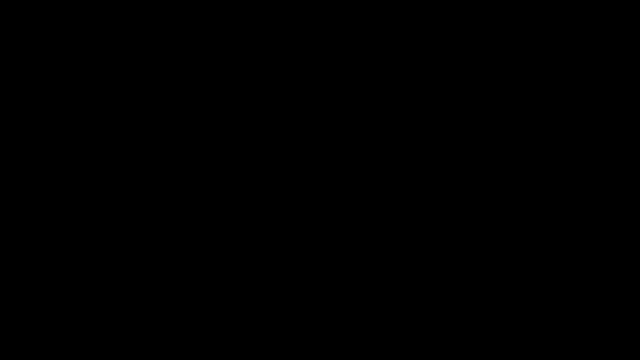 please be sure to leave a like and if you want to be notified when I post the rest of the videos in this course, make sure to subscribe. Thanks for watching.